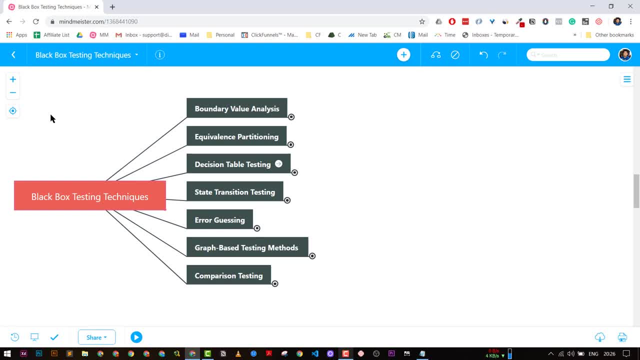 motive of these of these testing techniques. alright, so let me go, let me go you one. let let's go by one by one and try to understand this guy. this is the. these are the techniques that are going to help you in creating test scenarios, test cases, as well as these are the techniques that are generally 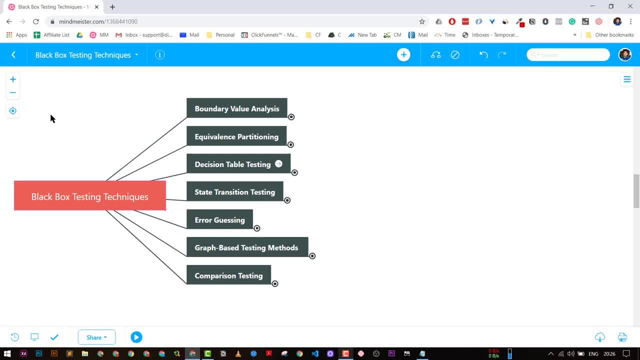 asked in interviews also, right. so if you guys are preparing for any kind of interview, this, these are the technique that you should know. all right, so let's get started. the first one is important one, which is boundary value analysis. right, so it basically means is that it's basically we are first. 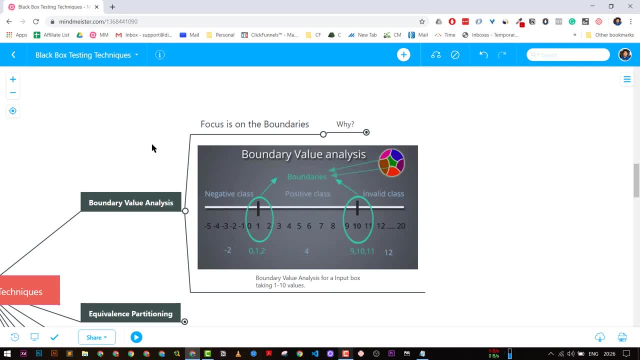 focusing more on the boundaries- of boundaries, right? so let me give you an example. for example, we have an input box, right, and it can take a value from 1 to 10, right? so what are the boundaries of it, right? so what we are doing here is: 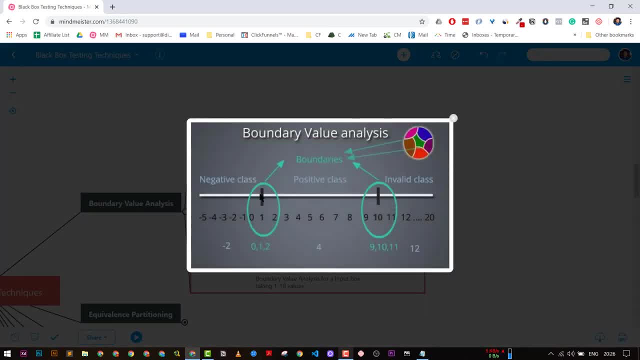 that let me zoom. let me zoom out here- is that the first boundary will be 1. 1 will be your, the first boundary and the start starting of the boundary, and the 10 will be your, the maximum value that it can take, right? so what you are going to do, 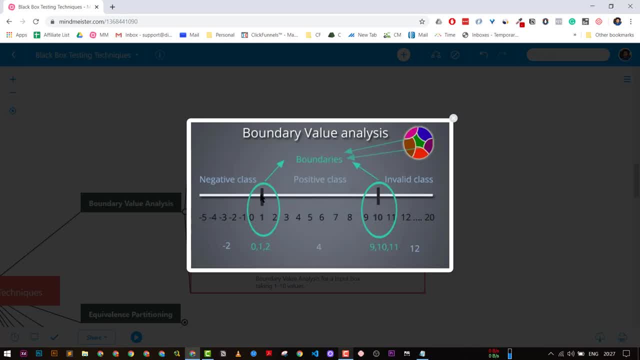 is that you the test case. whenever you writing the test case for this simple input box, how you are applying the black boundary value analysis is that you are going to put 0, you are going to put 1 and you are going to put 2. so these are the boundary of this system, right and 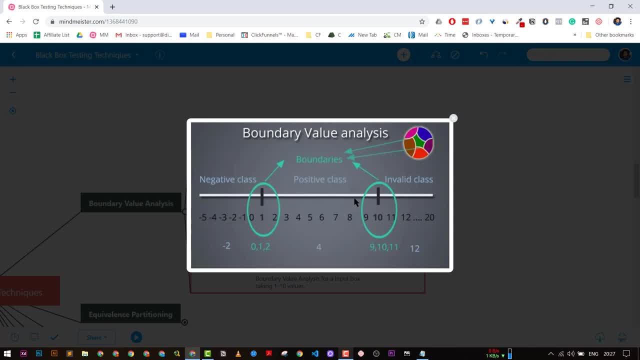 now, since these are the all positive killer, positive cases or I would say valid cases. so putting 1 or 2 value is just just checking out right means it will not give you much of the information, much of the bugs. but if you are going to check again with a 9, 10 and 11, then these are again the boundary. 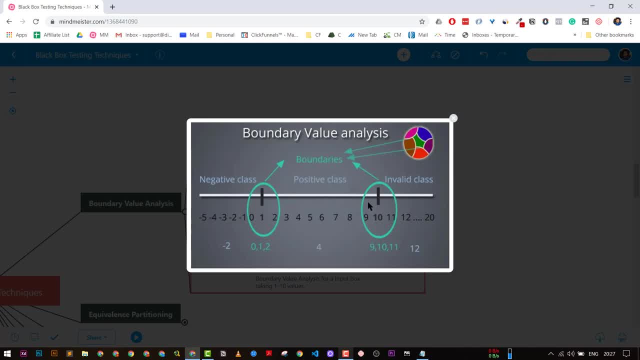 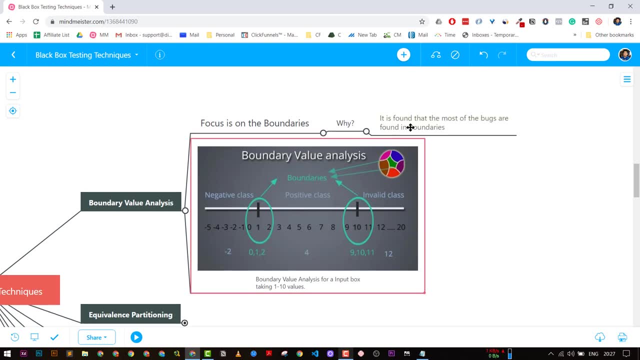 values where you will get the more like these boundaries are more prominent to the bugs, right? so why we are doing a boundary basis is that because it is found that the most of the bugs are founded boundaries, right? so these are the. this is boundary value analysis and 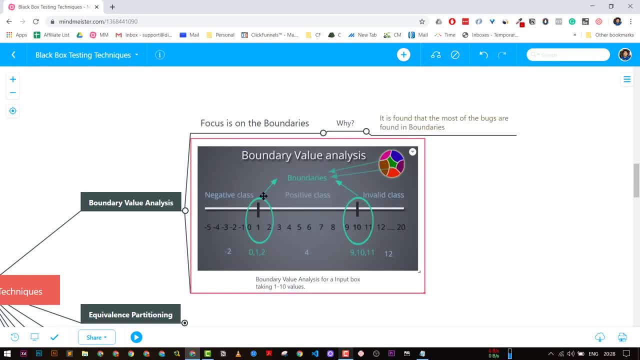 it's a type of a black box technique. we'll we don't know about the what is a black box? black box testing. it's a kind of a testing where we don't know the internal architecture but we know what is the input and what is the output of. 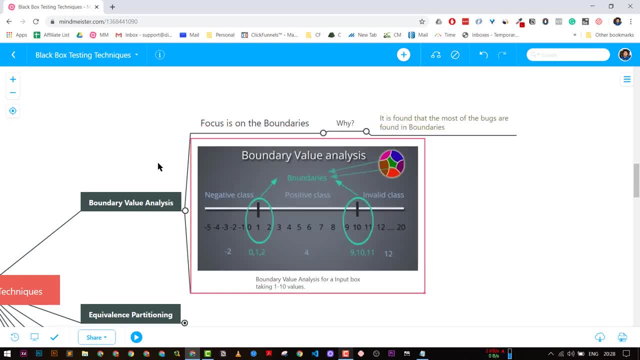 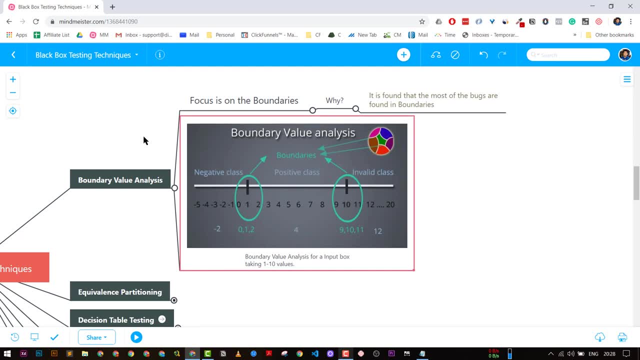 the system right. its basically an error, but we should know the internaly of the system right, because we努. so this is. this is the example. this is like a simplest example of any kind of boundary value analysis that you can apply. so let me give you another example. for example, you have a string. 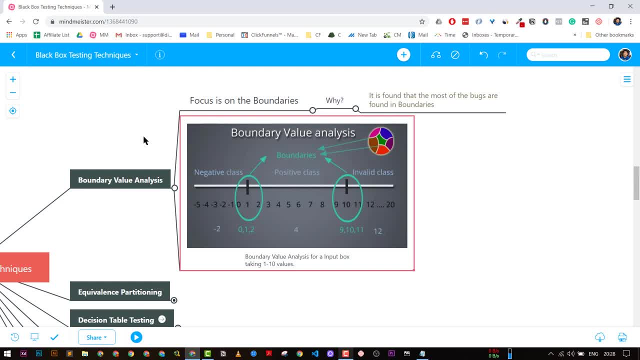 that you want. for example, you have input box where you can type a string with a maximum length of 100. now your boundary values will become any kind of null value, any kind of single character string and the maximum length of the string and maximum length plus one. my maximum length minus. 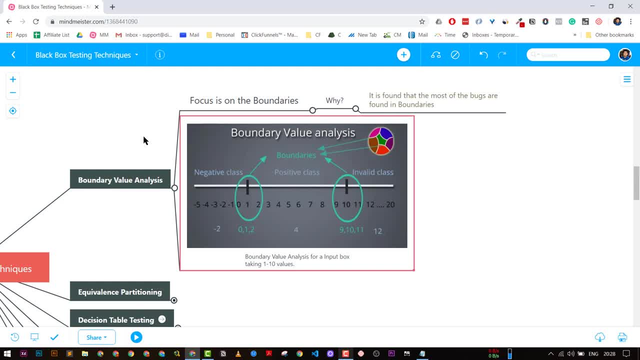 one, null, zero or no value. these are the boundaries values. right, these are the boundary values, plus some invalid cases. all right, these are not exactly the boundary values, but yeah, these are the invalid cases. most of them are invalid cases, all right, so i hope now you are able to understand clearly. 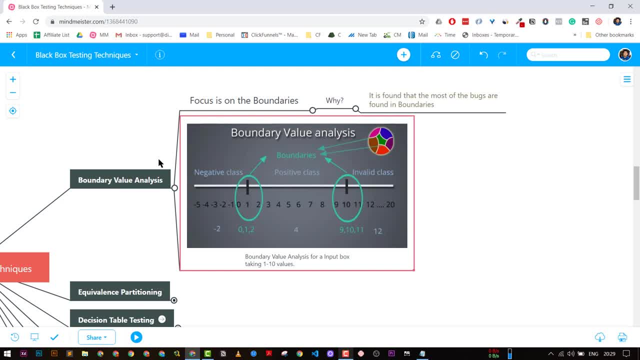 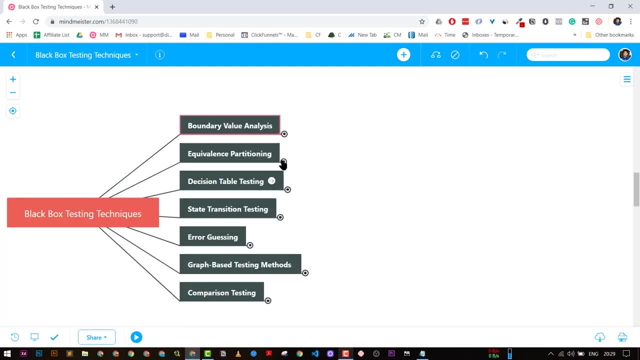 what is the boundary value analysis? right, so if any time any kind of interviewer ask you about this, you have to just give this example and explain it correctly. cool, now, this is the important one, uh, which is we call it equivalence partition, and lots of people don't. 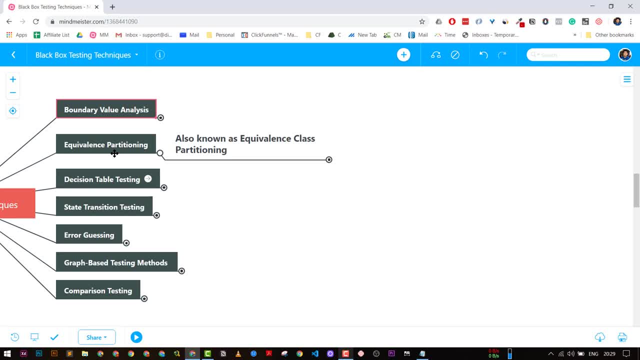 know about it and trust me, guys, whenever someone asks you that, what are the top, uh black book testing technique that you use. everyone knows about the boundary value, but lots of guys miss this equivalence partition. it's very simple, guys. it is also known as equivalence class partitioning. 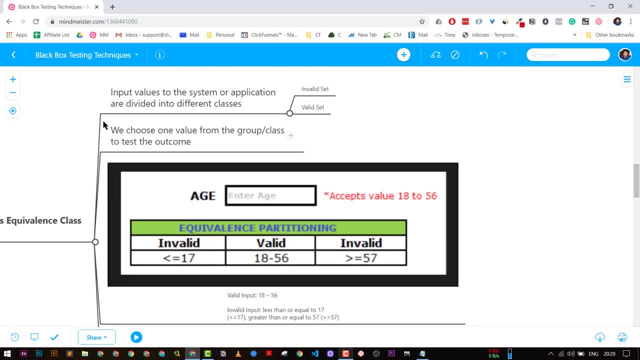 so what is it? let's start so. it's basically is a system. let me pull out my this one. it's basically: what you're doing is that you are input, input the value to the system or application, and we are going to divide the inputs into a certain different classes, right? so what are these classes? 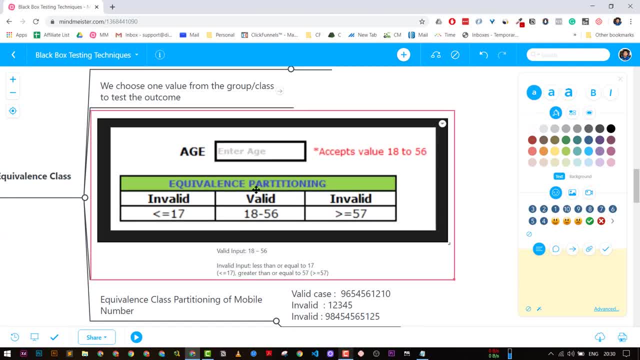 so, uh, what? let me give you an example, right? so, uh, this is again an input box which can take a age of a person, right? it accepts a value from 18 to 50 seconds. a wonderful example that is shared by someone. and so now what we have done is that we have created 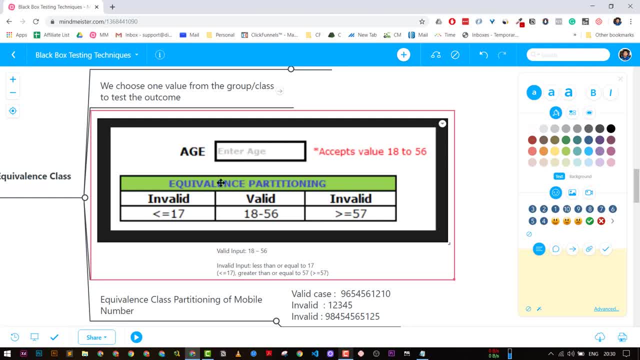 three, uh three, partitions of it. anything less than 17 is invalid partition, anything between 18 and 56 is a valid partition and greater than uh 57 it's invalid partition. so we have divided into three different partition. it's a very different from a boundary values where we have what we are. 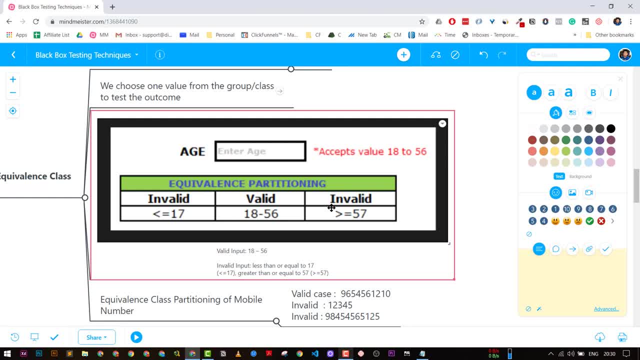 doing is that we were doing the bo. we are basically testing it for the boundary values, but here we are testing with a valid and invalid partition that we have created right, and uh, let's again, uh, take a simple example of a mobile phone. what we are doing is that this is the first one is: 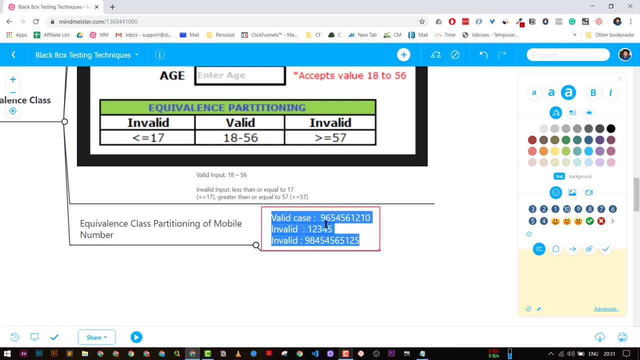 a valid number and inverted number can be uh whenever the number is less than the 10 digits, all right. and the valid in on the next set of invalid will be whenever we have uh more than the more than more than 10 characters, right, so we have divided into three. 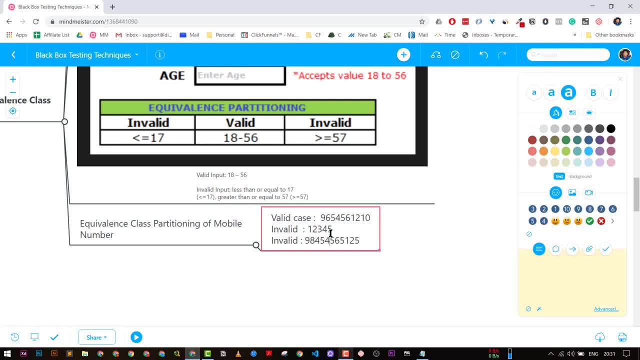 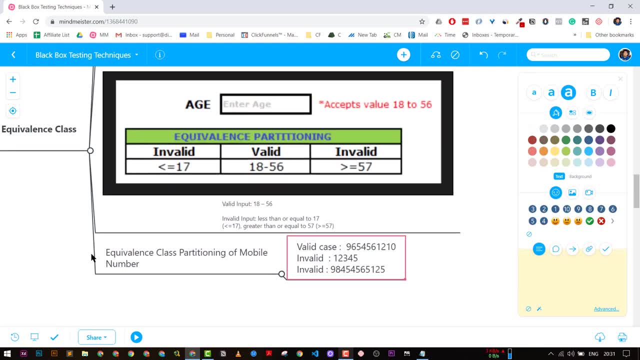 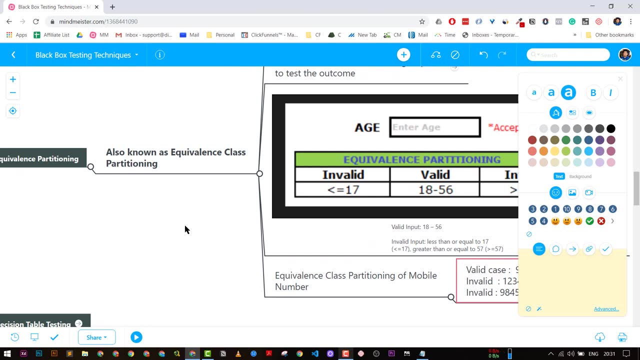 classes, basically two classes- valid and invalid- and invalid will have two more. uh, basically the lower invalid and the higher invalid right. so this is the equivalence partition technique. uh, you can say equals partition or equivalence class partition right, and it's again, it's a type of a black box. 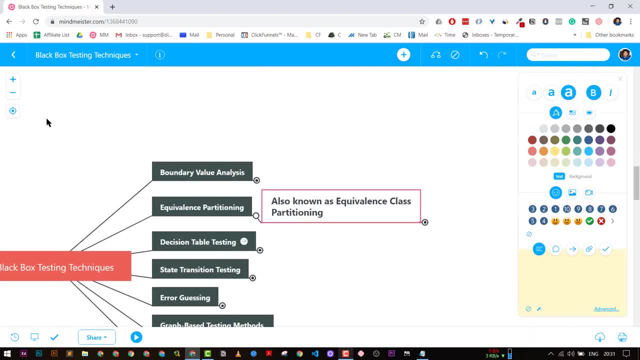 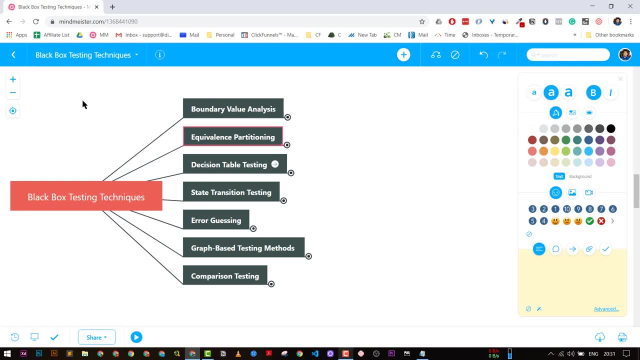 box testing technique. guys do remember this. and there's a huge, there's a great, i would say there's good, uh good difference between both of them. all right, boundary values: we are putting the boundary values equivalent partition class in. we are creating certain partitions of a class and we are 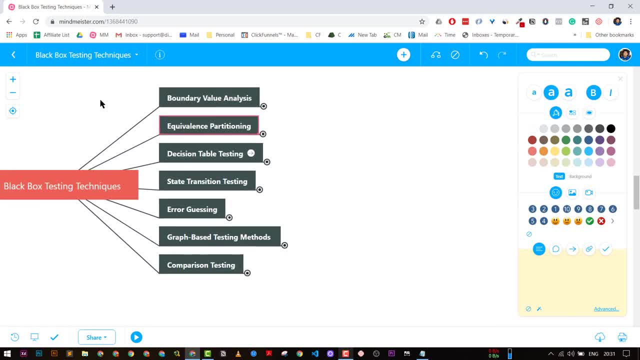 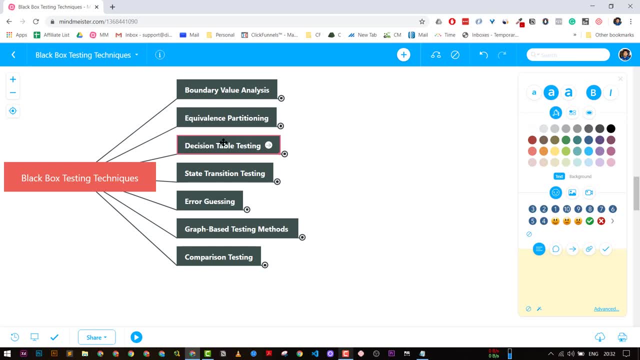 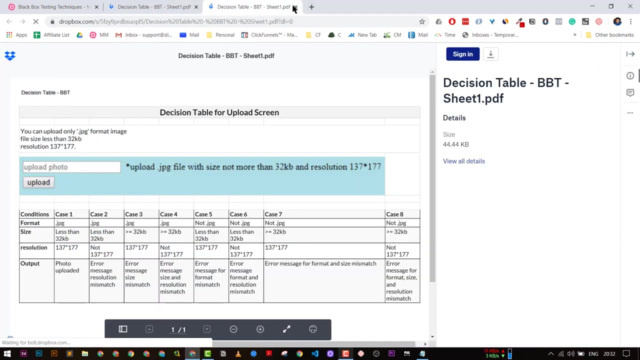 testing out that thing. cool, now the pro. the interesting thing starts here, when we have to uh discuss about the blackboard testing technique, which is decision table. right guys, let's, let let me open up a link and show you this example. let's, uh, let me show you this example. yeah, it's opening. yeah, you can copy this link and 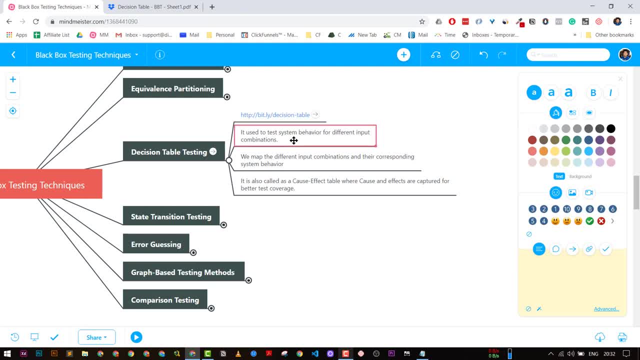 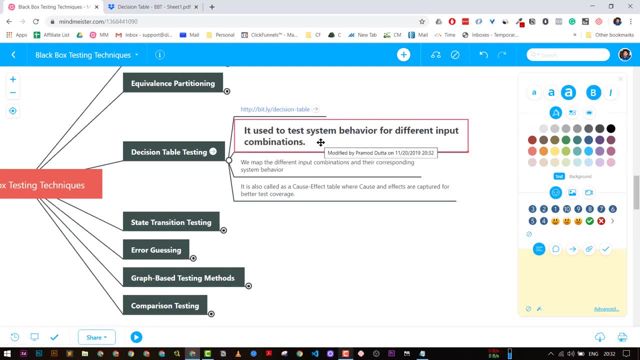 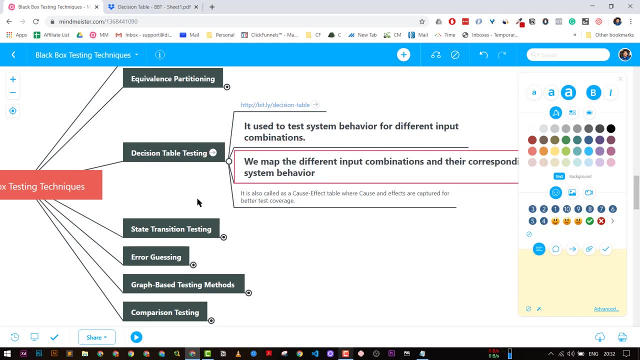 it's basically explain you everything about it. so it is used to test the system behavior for a different input combinations. cool, let me zoom out. what we are doing is that we are testing it for a different kind of input combinations. right, and we basically going, we are going to. 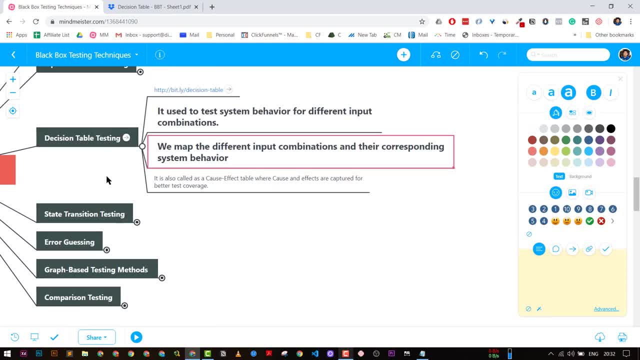 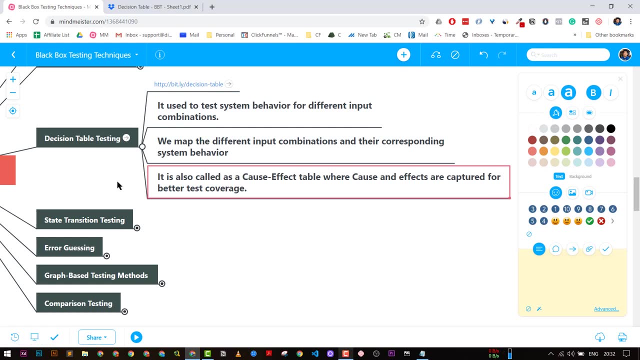 basically map the different input communication and their corresponding system behavior right. so different input combinations and their system behaviors. we are going to make a table out of it, right, and it's basically again. this is. another interesting point here is that it's also called as cause effect, where cause and effects are basically capturing in. 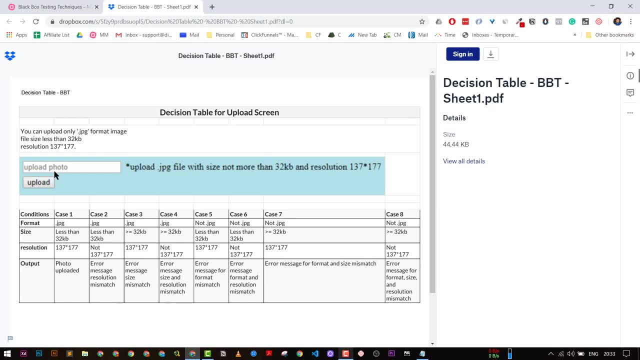 right saw that we have a better coverage. let's give an exact. let me give you an example so that you are able to understand it clearly. right, it's a wonderful example. suppose we have a upload photo functionality to test, right, and there's a button here- let me pull up my screen row here. so this is the. this is. 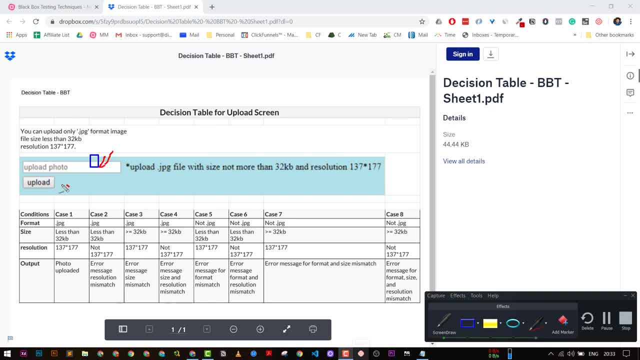 let me pencil. so this is the upload photo and this is the button. the interesting point is that you can upload only the jpg image. so the first constraint condition is that only jpg image. the file size should be less than the 32 kb. another condition- and the resolution is fixed. 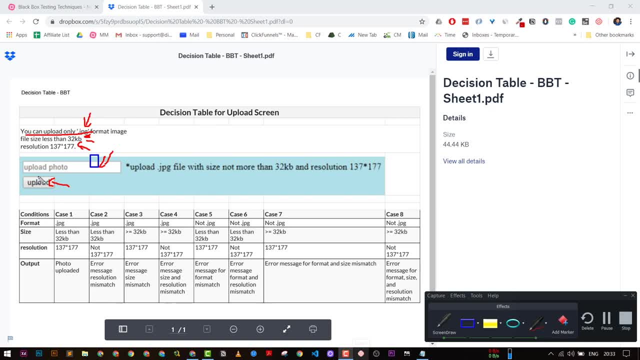 so we have three conditions, right. we have a condition of format, which is the jpg, we have a condition of a size, we have a condition of resolution and we have output- what exactly we are outputting? right? so the case one, what we are going to do, is that we are going to create a table. 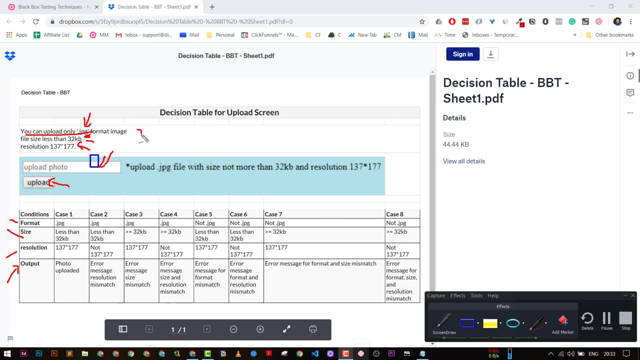 out of it, right, and if these are like three, three important conditions, and there will be two to the power. three, these are the number of combinations, which will be eight. right, and these are the. here it is mentioned, cool. the combination will be very simple: jpg, less than 32, same resolution. 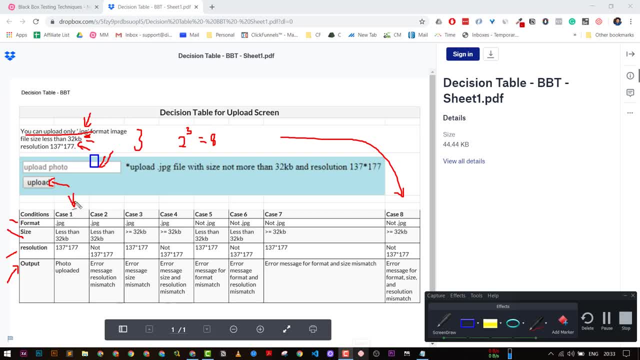 photo uploaded. this is the valid, this is the valid, this is valid. uh, you can say: well, it's an error, right, and most of them. these will be invalid scenarios whenever something is wrong. right, for example, if it is less than 32 or the resolution is wrong, the we will get an error if. 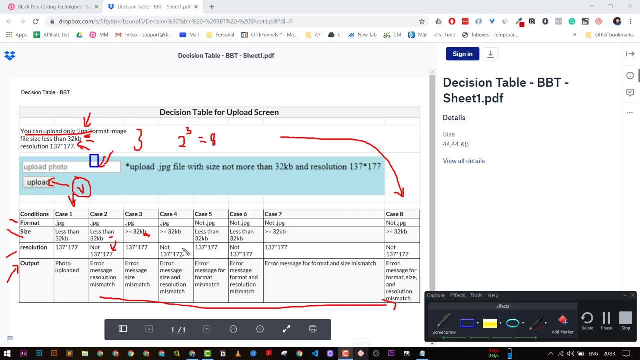 the size is greater, we will get an error. okay, right here the resolution again: it's a greater, we'll get an error. it's not jpg, it's not jpg, not jpg, not jpg, we'll get an error. so this is how you are. uh, basically, you have created. 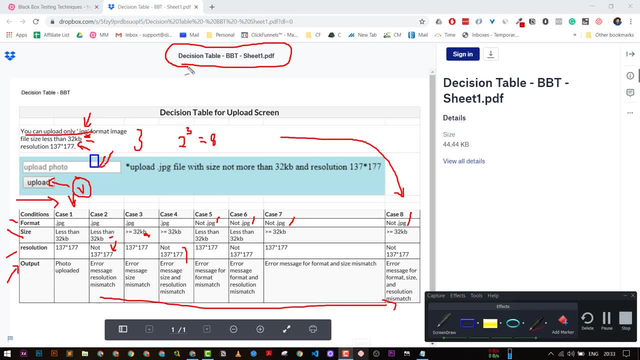 a decision table and it's again a black box, black box testing technique, right guys. so i hope you have got uh a great, immense value from it. and it's like the simplest example to explain you the decision table. so any, if anyone, if any of the uh interview, basically ask you about the decision. 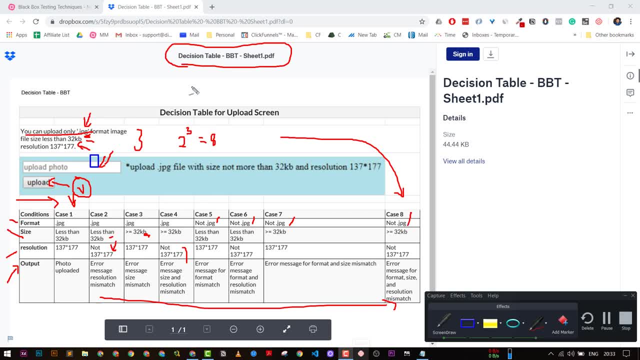 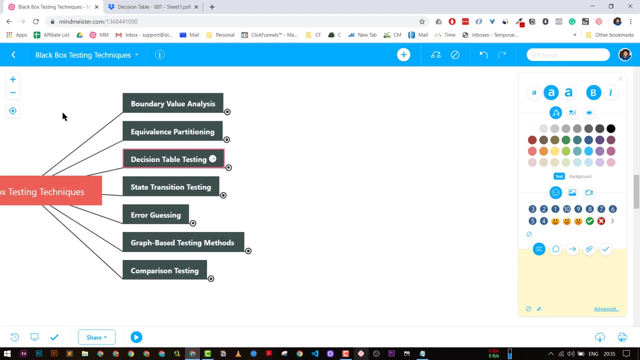 book testing technique. just give this example and you will. you are good to go, cool, all right. so let me. let's make it. give me one second, yeah, all right. so this is the decision table, right? uh, i know the guys, this is uh a long video, but you are going to get an immense value in this video, right? don't? 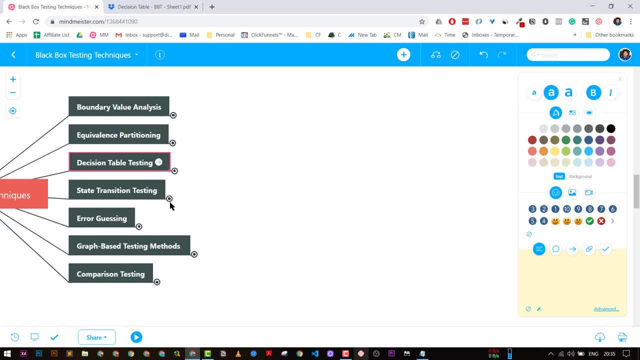 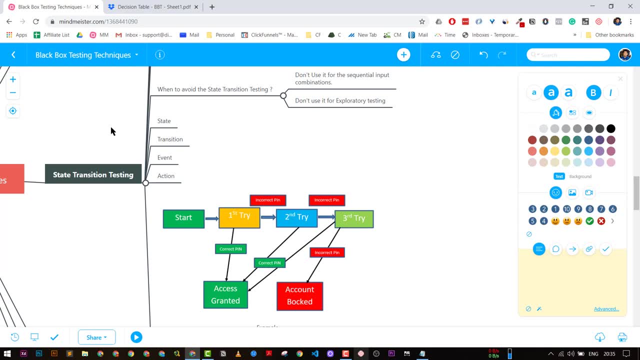 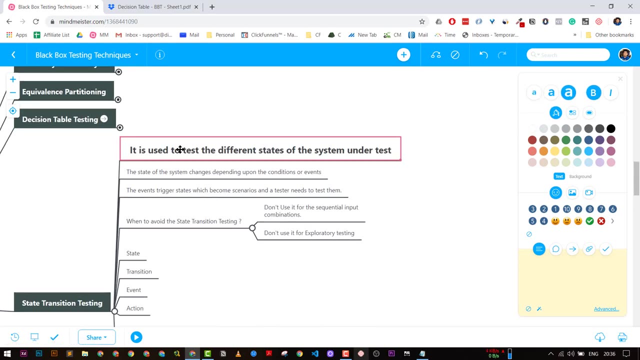 just, uh, watch this full, full tutorial so that you get the knowledge about it, right? so, state transition- again, it's a black box testing technique and what we have is that. let me show you in a simplest way. uh, it's. it is used to test a different states of a system, right we? 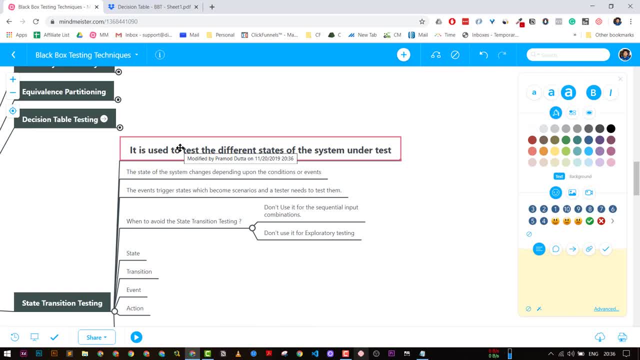 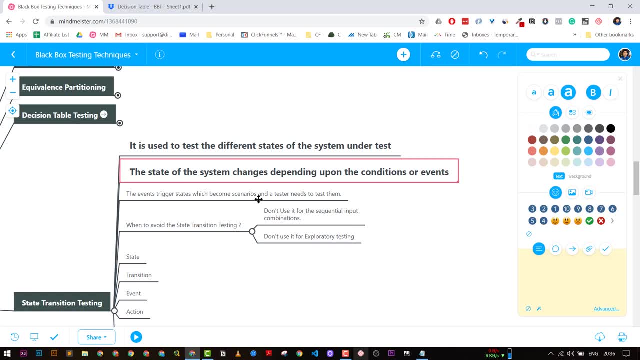 are majorly concerned about this different type of states. we have right. the states basically means is that the state of a system depends on the conditions, right? uh, i'll give you an example so that you can understand betterly, uh, better, and i'm going to share this uh full. 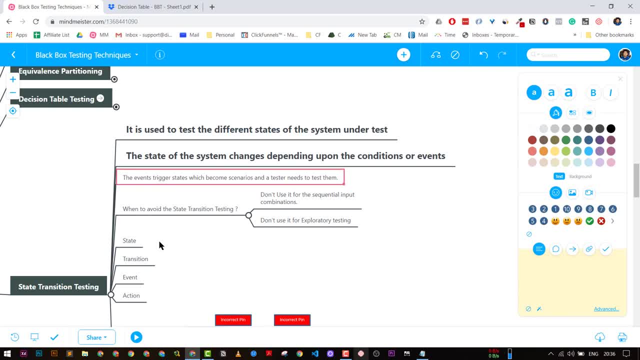 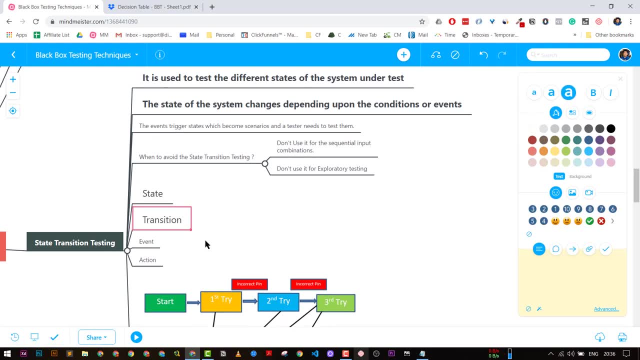 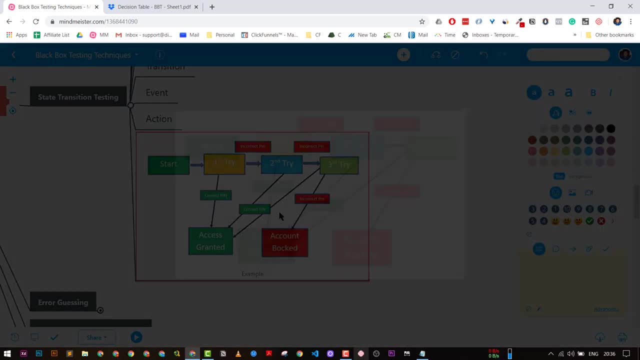 mind map with you, don't worry about it, and we have. uh, what we have is that in the state, transition testing is: we have a state, we have a transition, we have an event, any kind of event- and we have an action. these are the four things. so let's take an example of this one. this is very interesting arti. 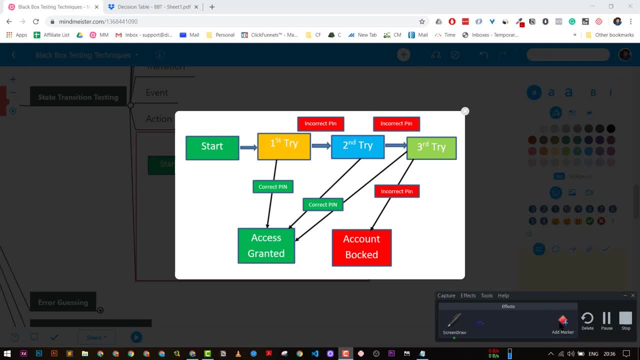 uh, die, uh, you can say: screen draw, let me pull up this. yeah, so we are starting. this is a flow and these are the states. basically, we are going to first try. this is, you can say, an atm machine and we are entering a pin. so we are doing a first try. this is our first state. 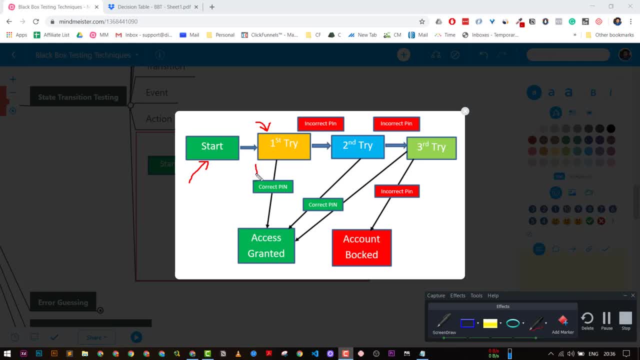 and after that, what we have done is that we have the entered our pin. that is our action, that we have, and the tradition is that if it is a correct, we are granted with access, but if we have incorrect pin we have, we are in a second state. 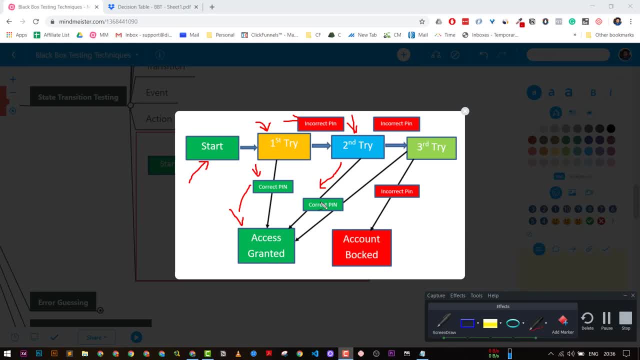 the second state. if we put correct uh pin, then again we are access granted. but if it is incorrect we are in the third try, and if third try is failed, incorrect we have, then we are, our account is blocked right. so this is, uh like a different states. 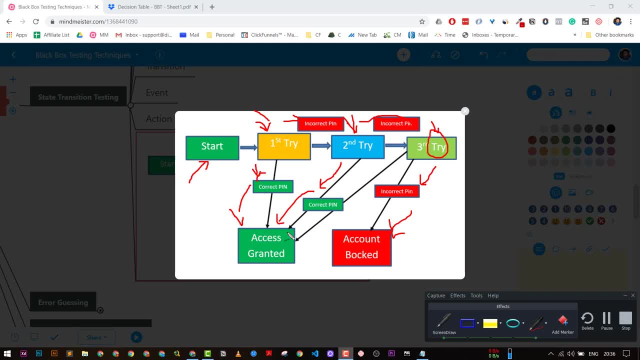 different actions that you have done and different uh events. that has been occurred whenever you are doing different kind of uh, whenever you are putting a correct or incorrect step according to it. so you can, you can do it in different ways according to it. cool, so i hope uh. 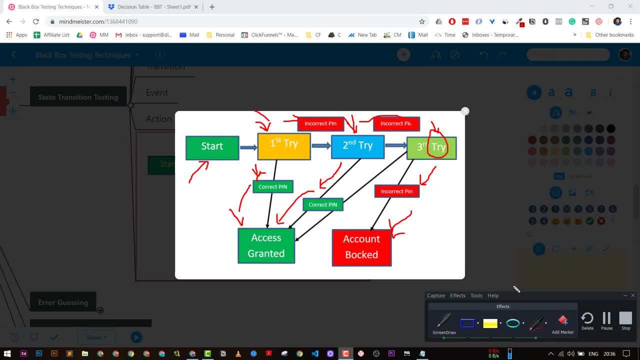 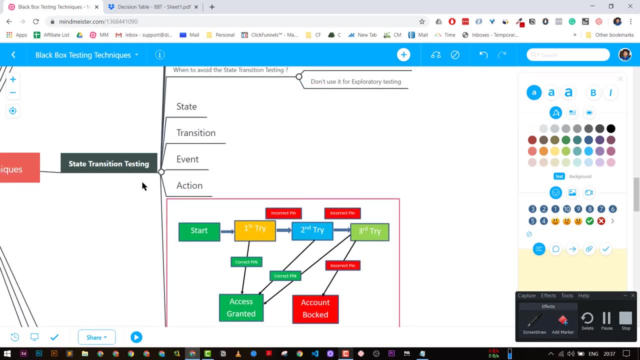 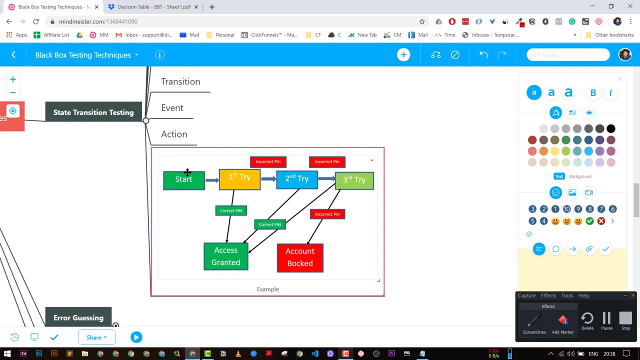 that is very, pretty much clear about it. it's a very simple example and it, whenever anyone basically basically ask you about this one, just give this example and you are good, uh, good, to go right, state transition testing is simplest. uh, very simple. you have states, you have actions, you have 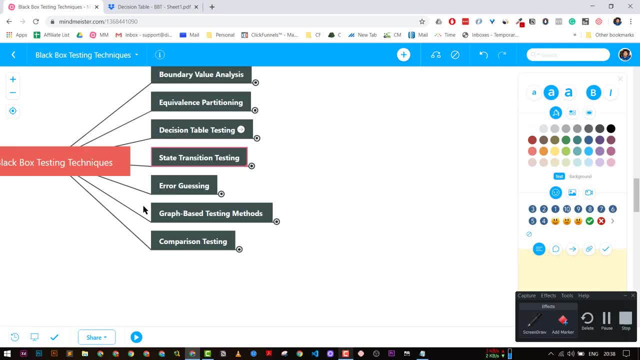 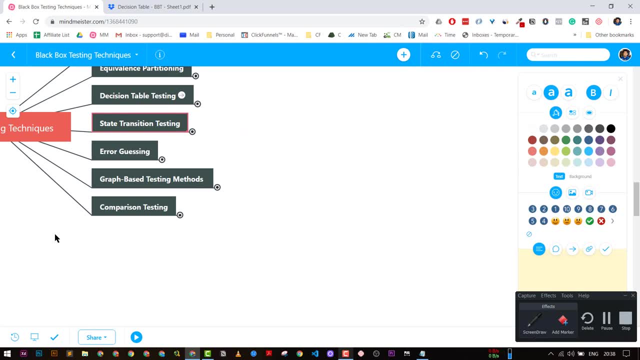 transitions from different state to state and you are going to take a action, cool, all right. so, uh, of last three ones- and these are important, important. i know this video is going to- uh, you're going to get a great value in this video. uh, error guessing is very important, guys. it's a. 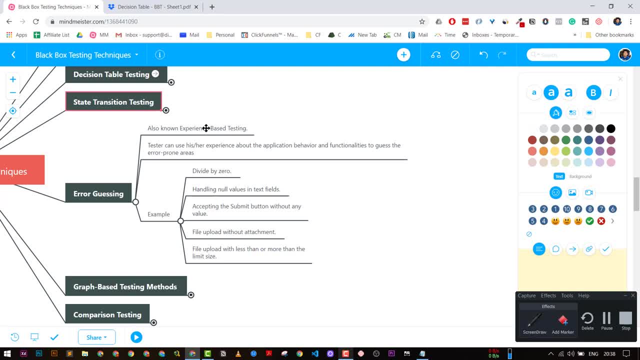 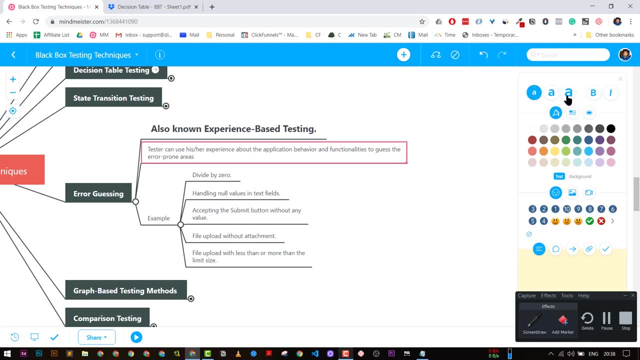 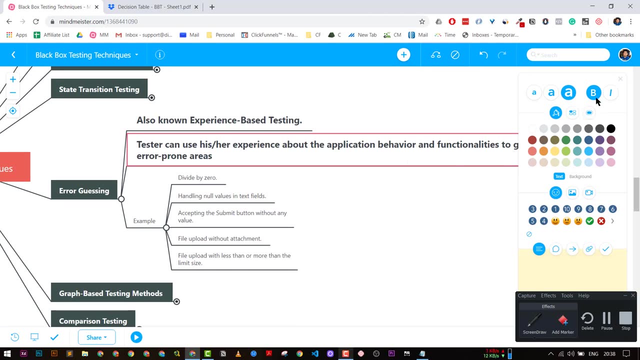 very simple, simpler black box testing technique. what you do is that it's basically called as experience based testing guys. so what you do is that, uh, generally testers can use or uh, his or her experience about the application of behavior and to guess the errant prone area. 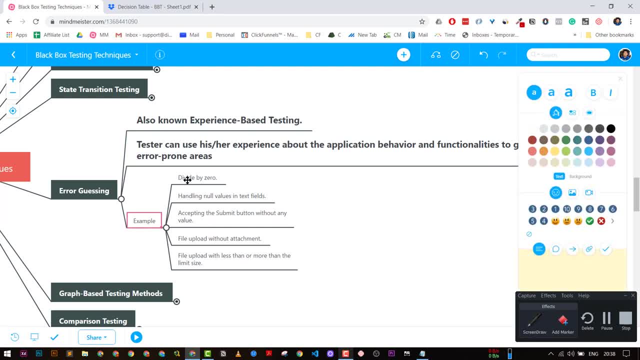 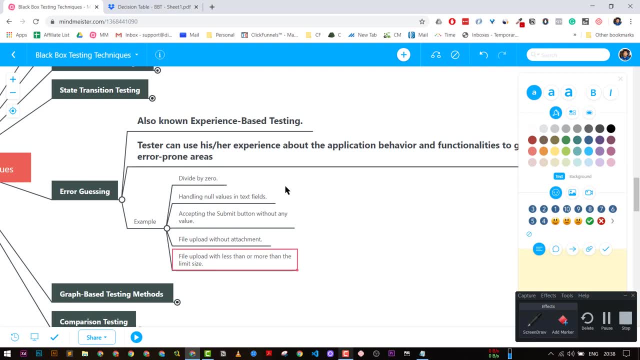 so, for example, it's very simple: in one right, uh, we can check for divide by zero, null handling, submit button not working file, not uploading. these are the error guessing. we are just guessing that this can be an error because, uh, it is due to the experience that we have already. 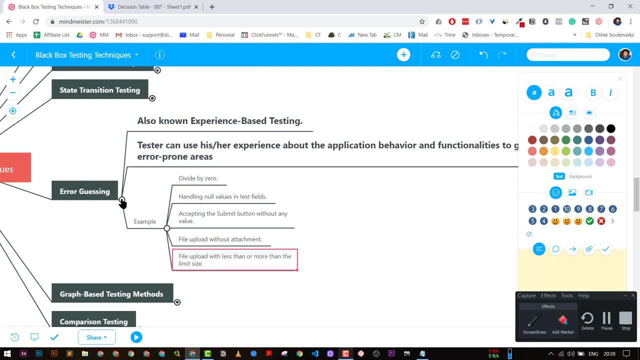 right, so it's very simple. uh, i don't have to give you much of example in this one, but just you can see that it's very simple, right, so it's very simple. uh, i don't have to give you much of an example in this one, but just to. 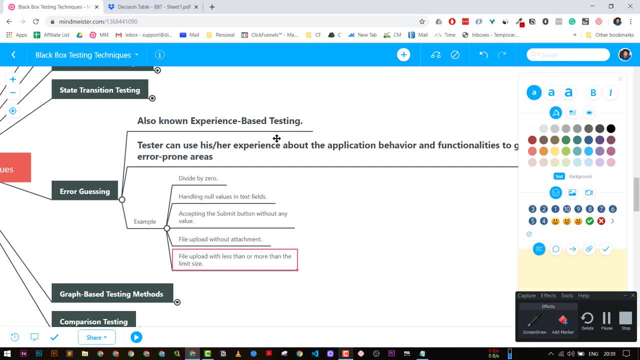 make- just remember it's experience- by testing where we are just uh, basically, uh guessing the uh output, uh guessing the error prone areas and, for example, we are doing divide by zero if it is in certain calculations, we are checking for null values and different file uploads, something like. 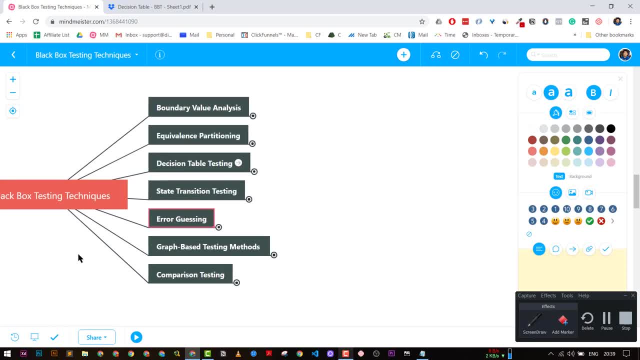 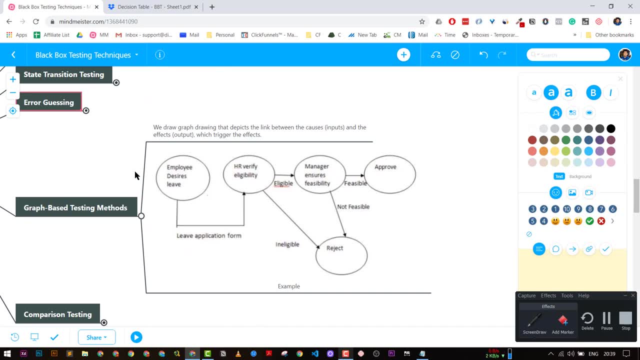 this all right, cool, uh. now the interesting part, uh, which is graph based testing. it's again a very interesting type of black box testing. what we do is that we basically create a graph. we draw a graph by depicts the link between the cause and the effect- again, the concept of cause. 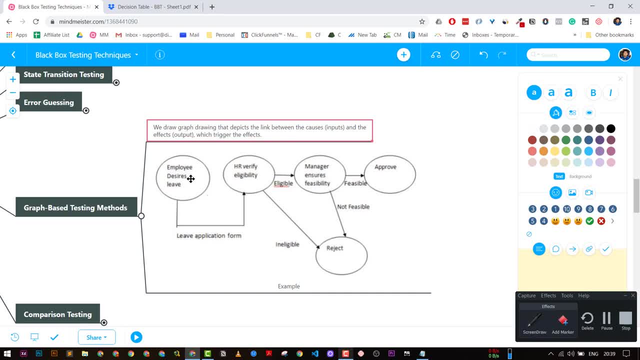 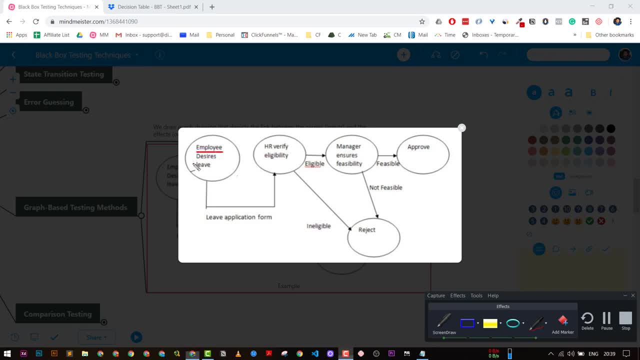 and effect. it's basically an input and output. so, uh, this is an example. it's very great example. again, let me screen to a screen draw. we have employee which desired, which basically wants to leave, so this is a graph, basically. so this is, this is how it go, and 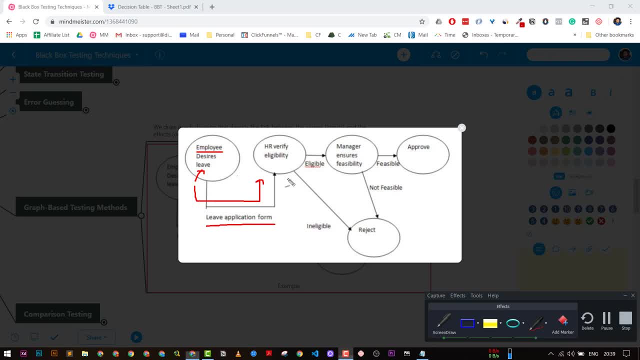 he basically try a leave application and it can have two inputs: outputs right, hr verify if it is illegal or not not as a label right, and after that uh manager will ensure the feasibility. if yes, if not visible, reject uh. if hr has uh basically rejected, then it will also reject it. if manager. 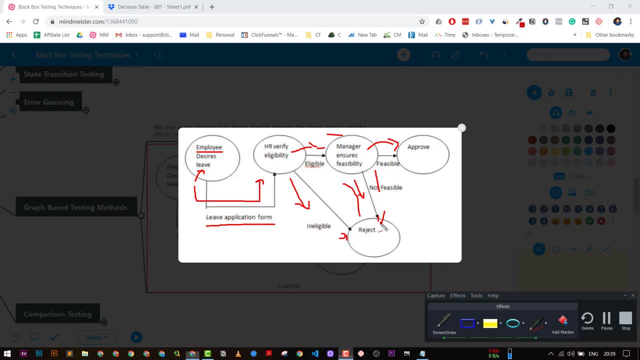 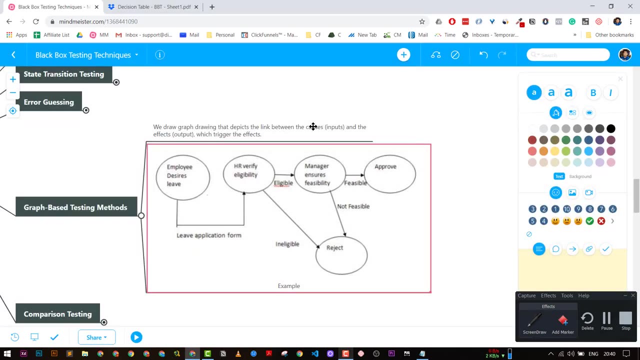 allowed it, it will be approved. it is not, then reject, right. so it's a graph basically going from here to here. you can go to here. these are like certain cases that you can, right. so this is called as graph based testing, where we have a graph links between cause and the effect. guys, just remember that thing. cool, all right. 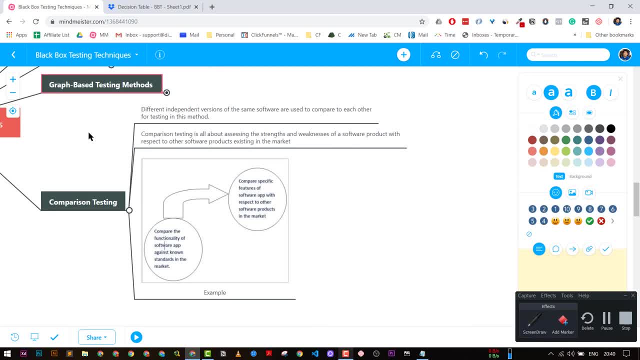 uh, the last one is comparison based testing, which is very simple, very simple. it basically means that we are different input, different independent versions of the same software are used to compare each other on a testing method. so basically, what you are doing is that, for example, you are testing- um, let me give it for example- you are testing a. 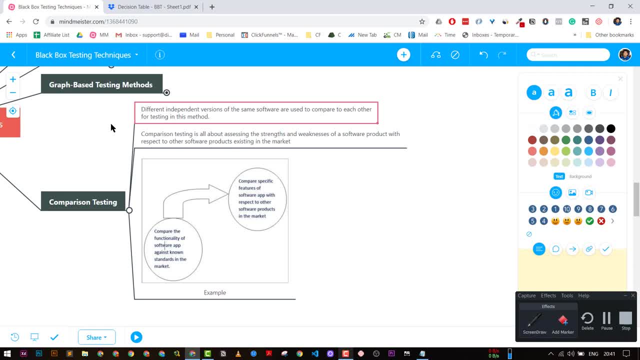 gmail application. so similar application is hotmail app, right? uh, we have a gmail alternate as a hotmail, or you can say outlook, right? so you are going to compare the features here, and comparison is all about accessing the strength and weakness of the software, for example. we are going to 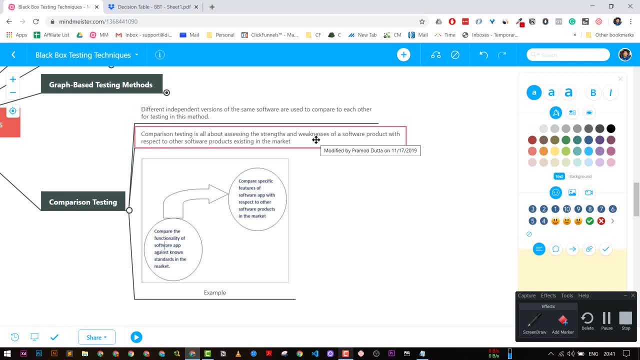 check for strength and weaknesses for gmail, and it is our level on our, So that is also a kind of a testing right, And this is known as comparison-based testing, which is a part of black box testing. all right, So this is a simple example.